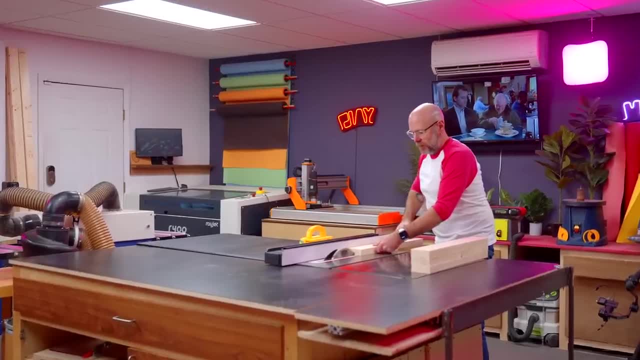 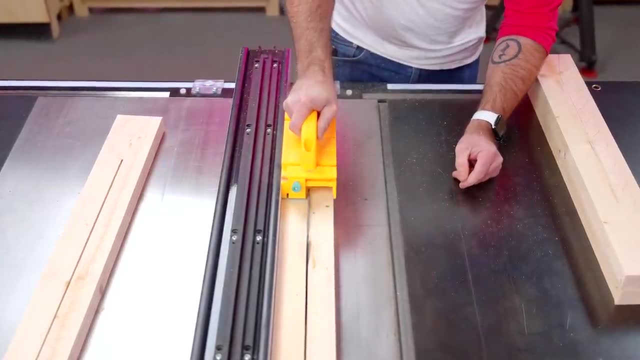 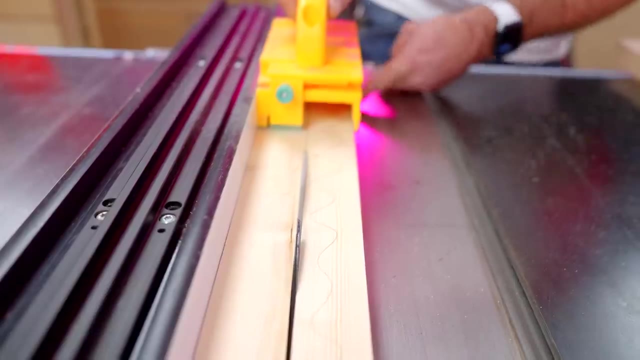 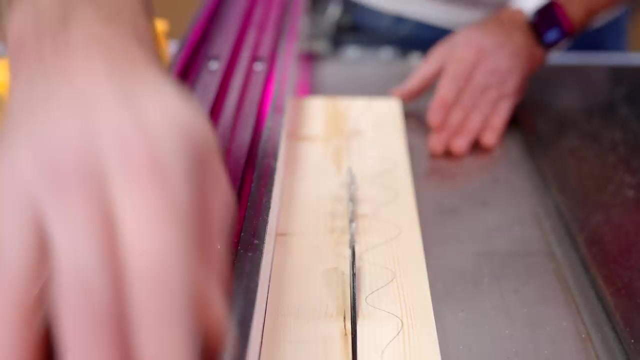 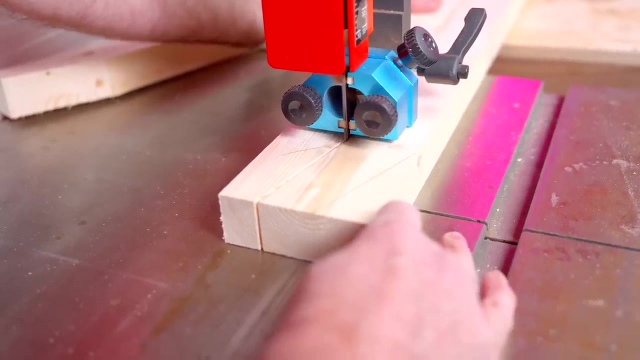 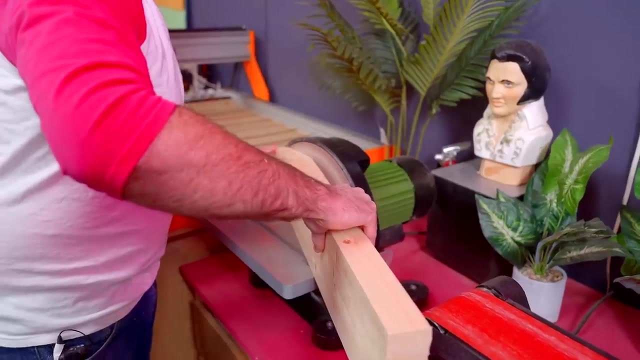 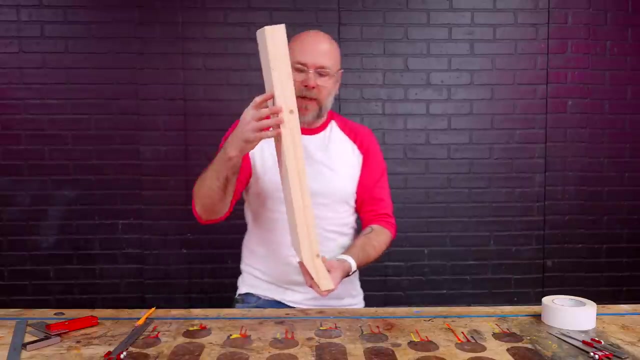 off Over on the bandsaw. 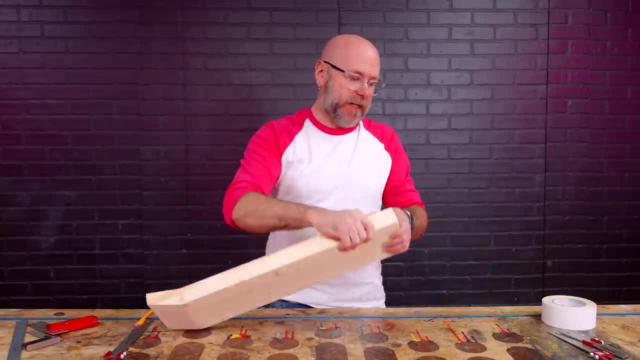 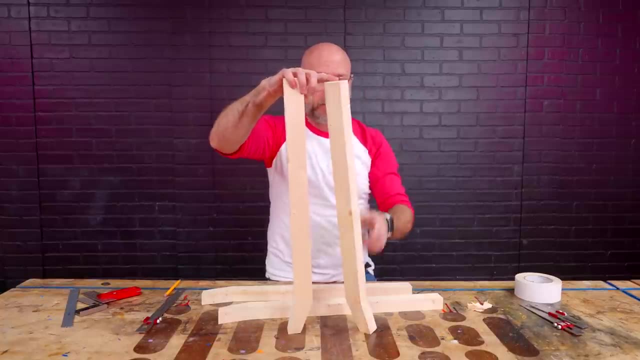 They all came out exactly the same shape and size. There'll be two legs up front, two legs in the back. Now I have to go to the table saw and cut a groove that's going to hold. 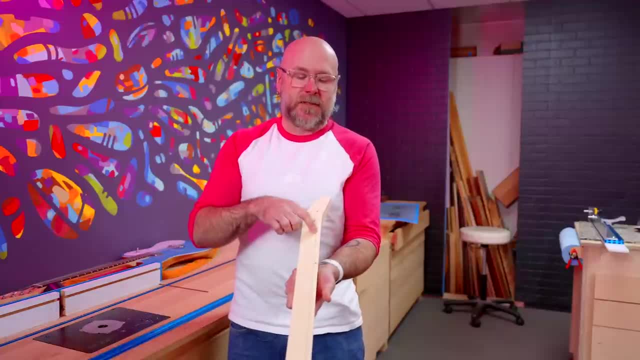 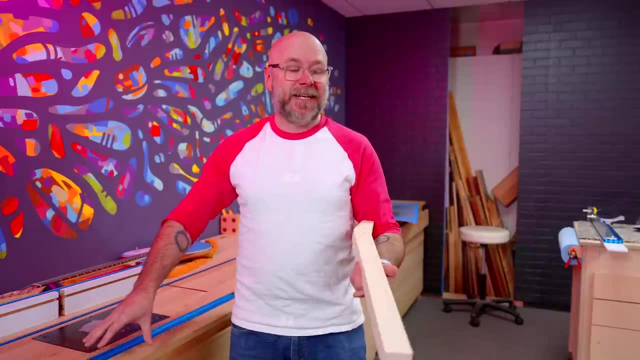 the sides and the back. I said I was going to cut this dado over at the table. saw I changed my mind. The router is a better tool for this operation And I just changed my mind again instead of doing any of that. 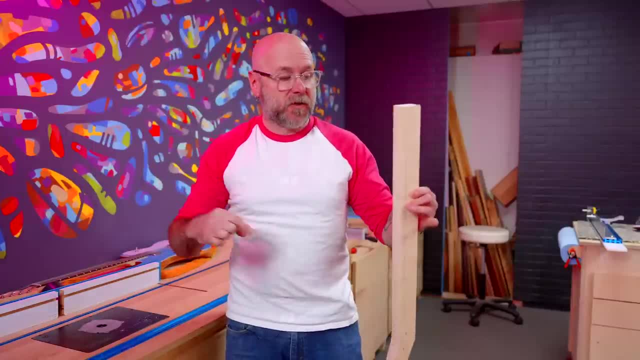 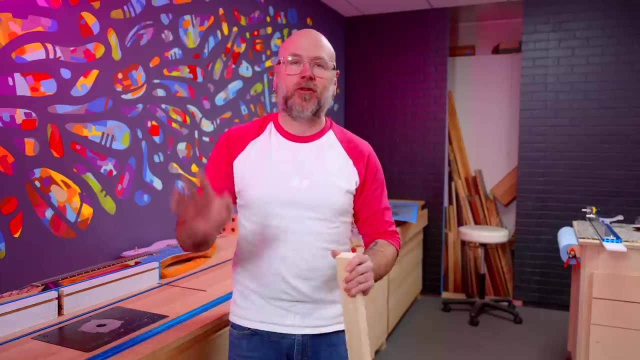 I think I should cut the rails. That's going to go all the way around this first Cause. that's going to help me with the measurements. So stop changing your mind and start cutting. I get a lot of comments Like: you talk too much. shut up and cut. You talk too much. 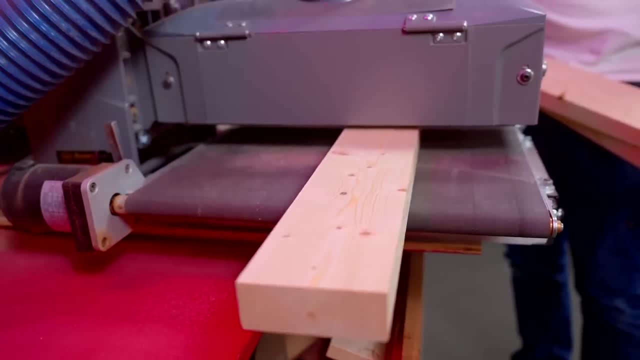 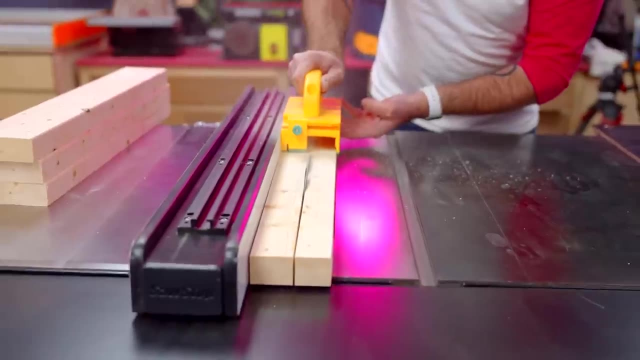 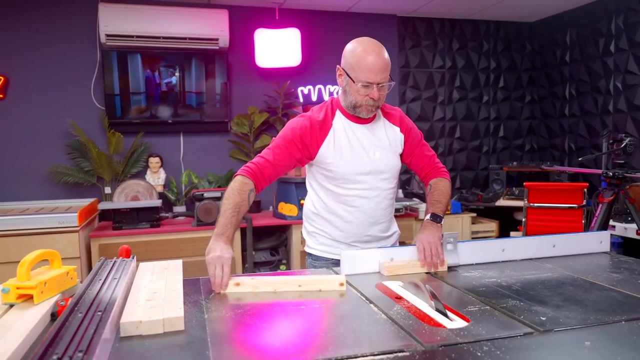 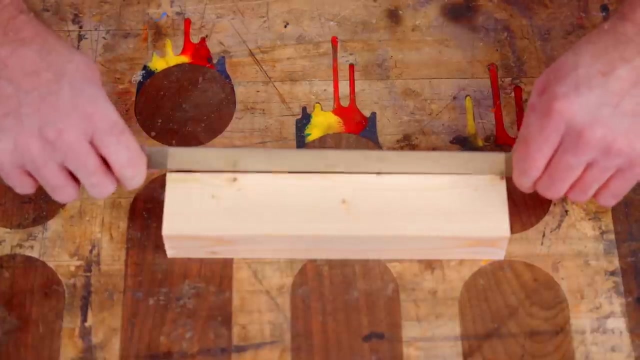 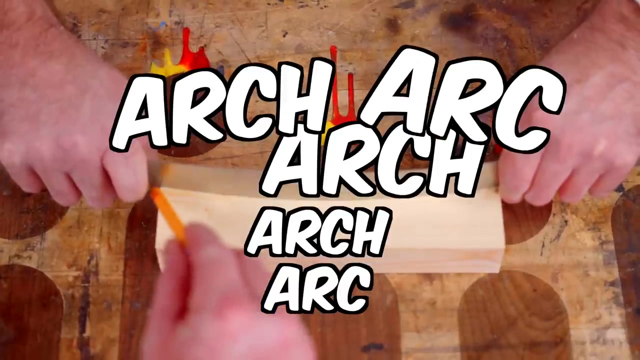 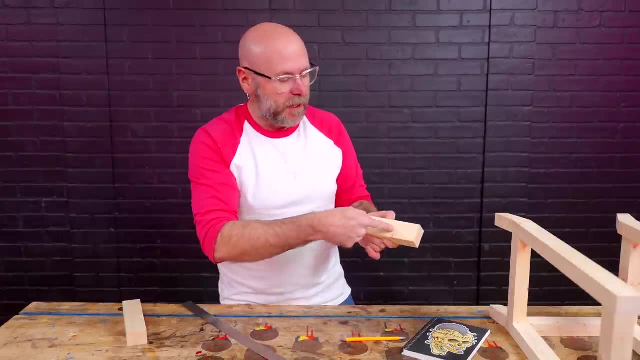 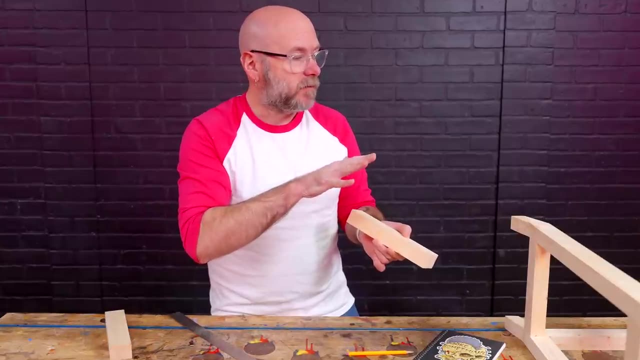 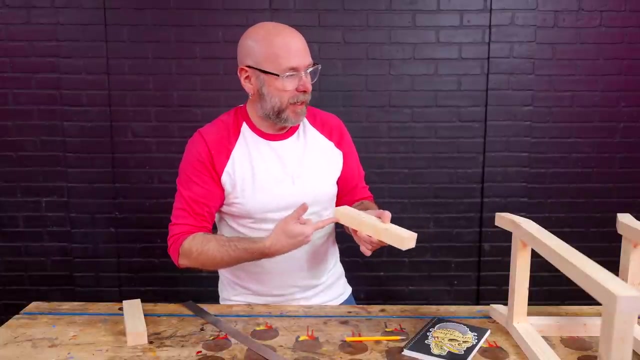 just decorative, just to make it look fancy. So before I cut that arc out, I want to cut a dado on the bottom of all these, except for the front pieces, Just kind of figuring this out as I go um. the hold the sides and back panels. 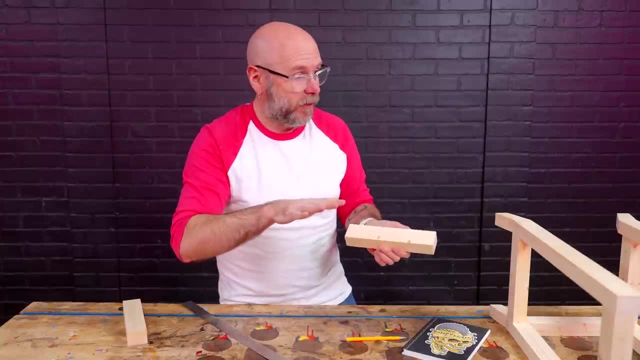 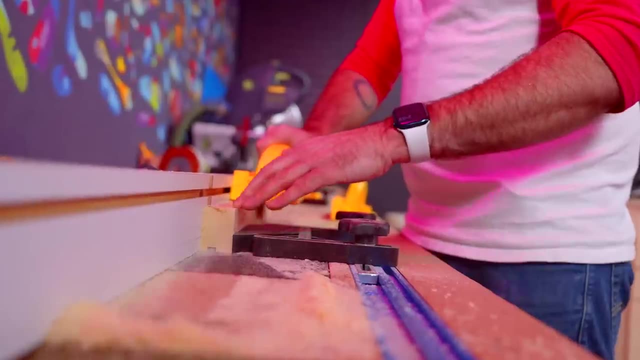 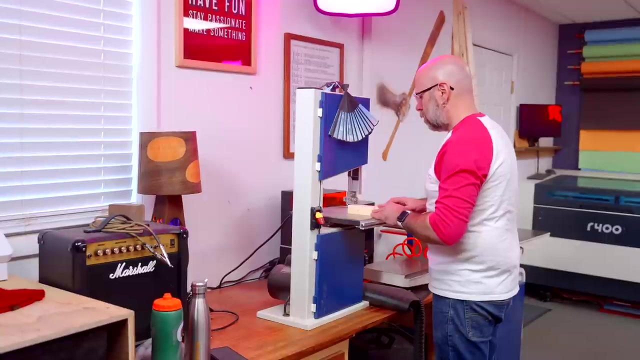 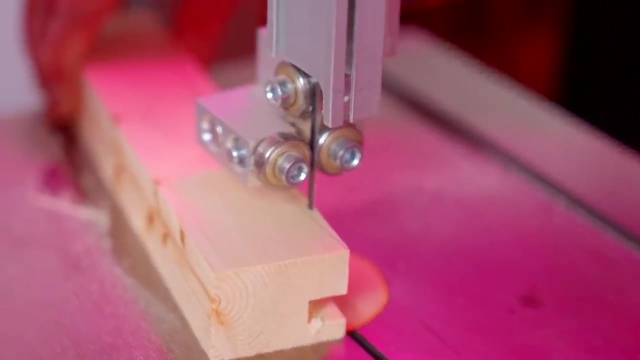 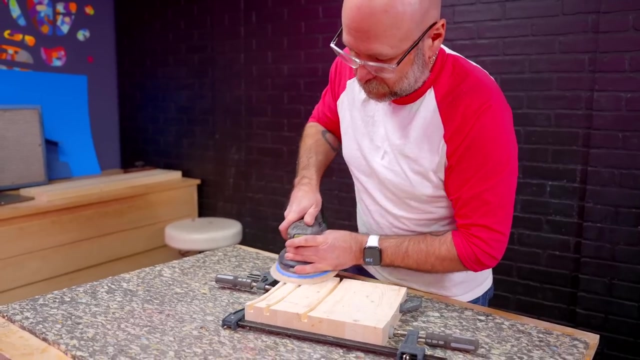 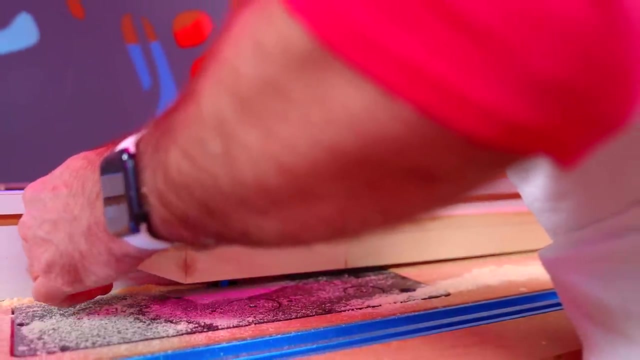 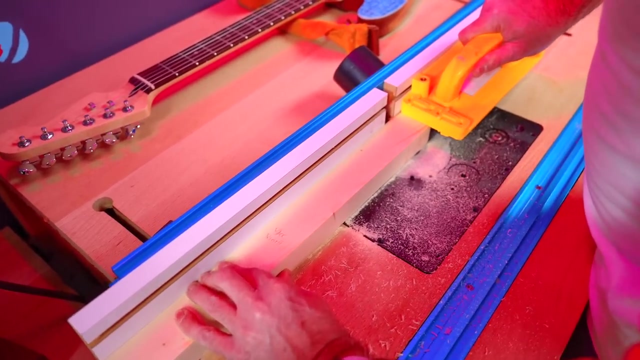 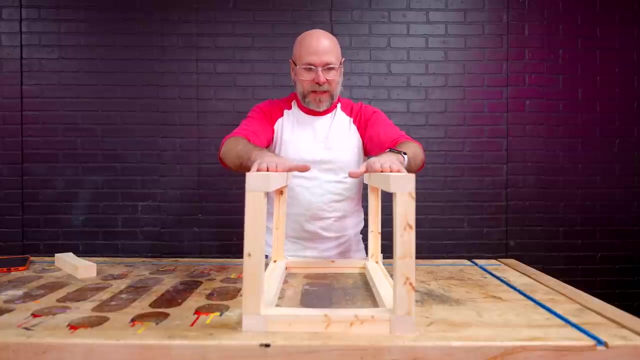 I got to remember to not cut too many, cause there's not going to be a front panel. I've got, I've got a plan for the front, As long as I don't fuck this up. I've got everything kind of rough assembled here. 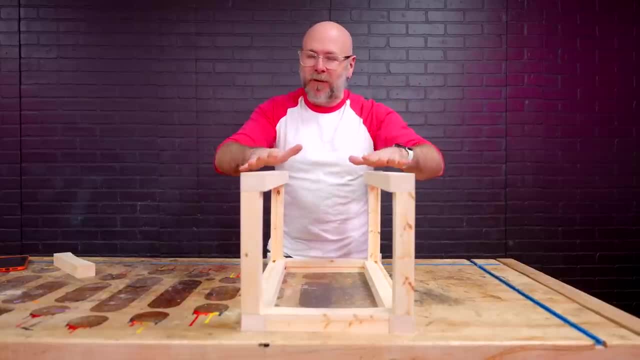 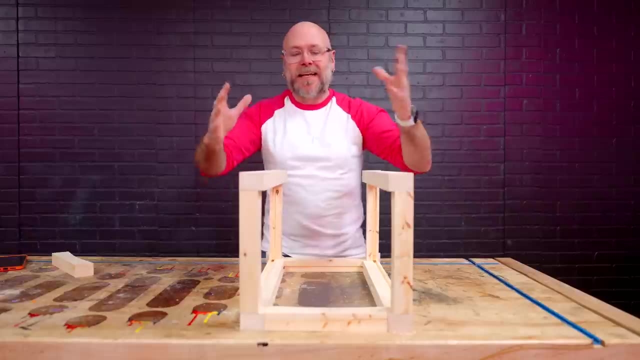 Now it still might look a little bulky. and two by four E take it easy, Take it easy. I got a plan. This is going to look really good. This is one of like, the cool thing about this is normally a lot of times we're 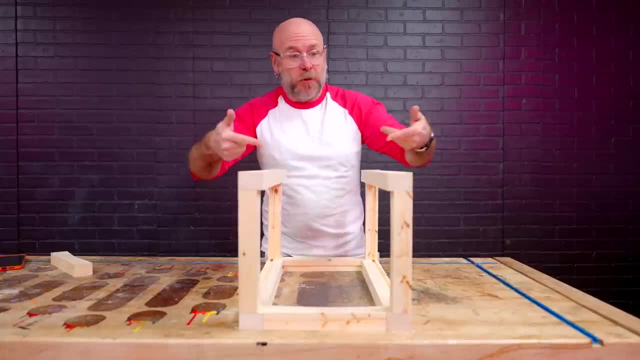 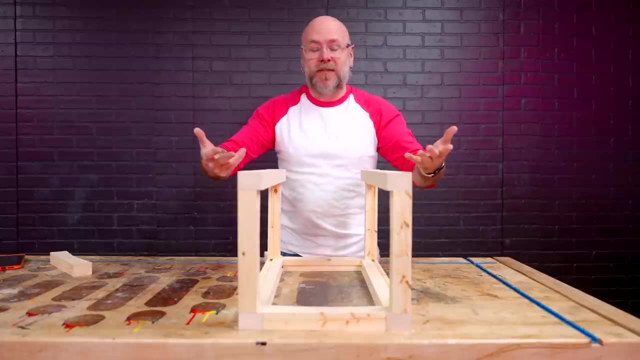 just working with three quarter inch material. because we're working with inch and a quarter material, We get to play around with different looks, And if I was going to use inch and a quarter walnut for this, this would be kind of an expensive project. So I am really happy. 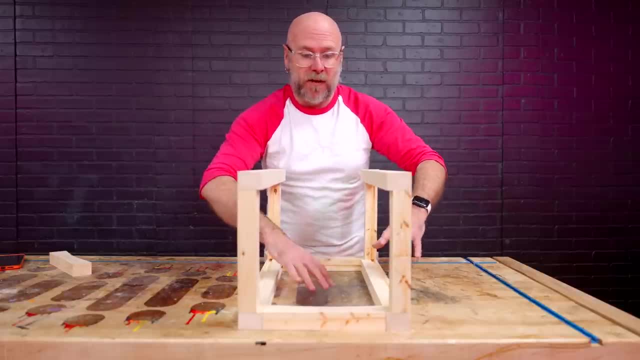 I think this is going to look really good, So I need to make the three panels that's going to go in the back and the sides and they're just going to float within these grooves And the reason they're going to float in there is 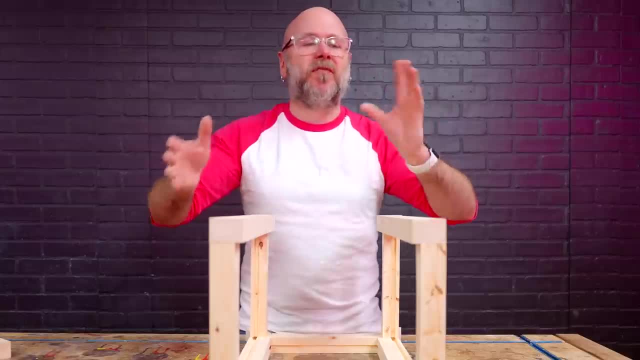 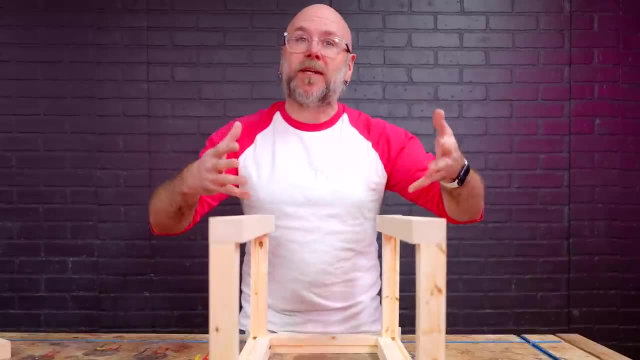 is because it's going to expand and contract And this stuff wasn't dried properly, or at least not dried to fine woodworking conditions. So these boards are going to move quite a bit, So I just want them to free float in these grooves here. 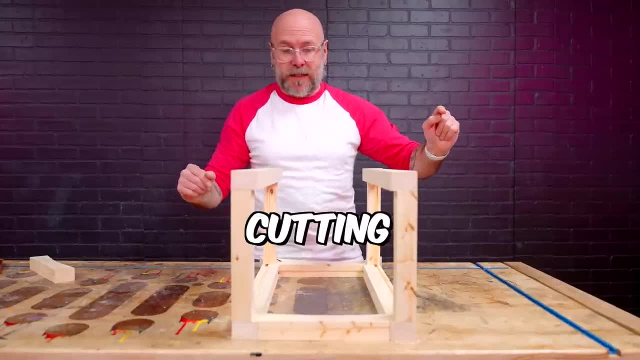 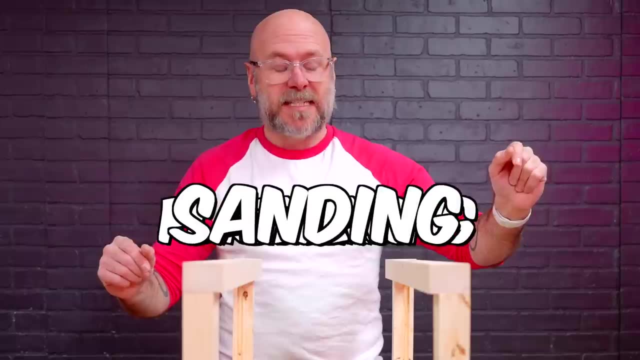 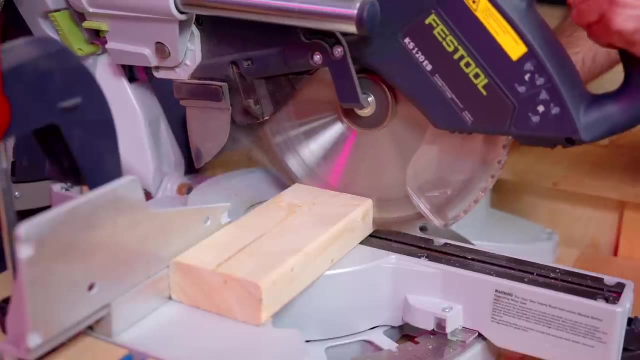 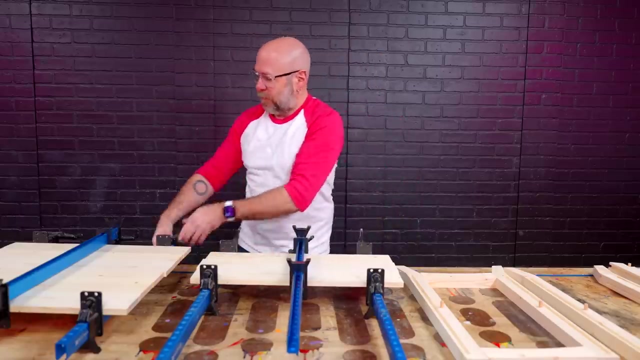 So back to some two by fours: cutting, resawing, gluing, flattening, sanding and cutting in that order. Now we're going to glue up these panels. So these have been sitting in the clamps for a few minutes. 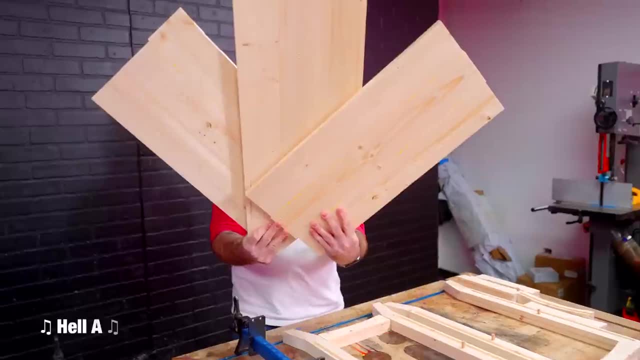 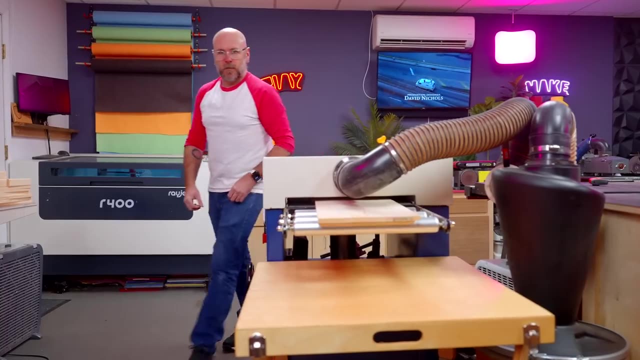 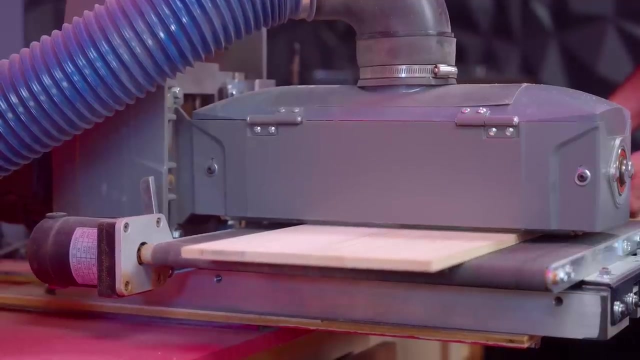 We're going to take them out and plane them down, And then we are going to glue them up here and then we are going to add our body to the frame. These are already in real-time Here. back here, we want to do it a little bit more. 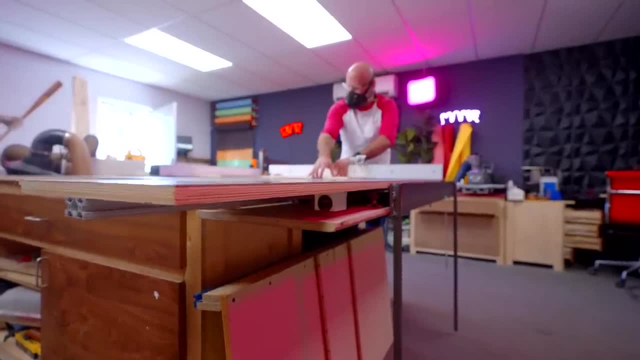 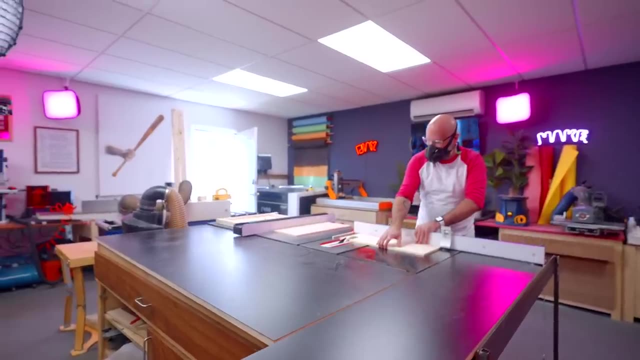 I need to get it to seem a little bit more solid. So I'm going to do this side first. Then I'm just going to have to put it in this press pipe Here. this is where the soldering should go, Alright, so we're going to go ahead and do that. 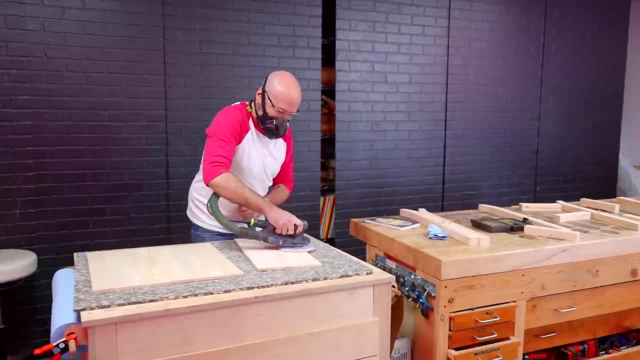 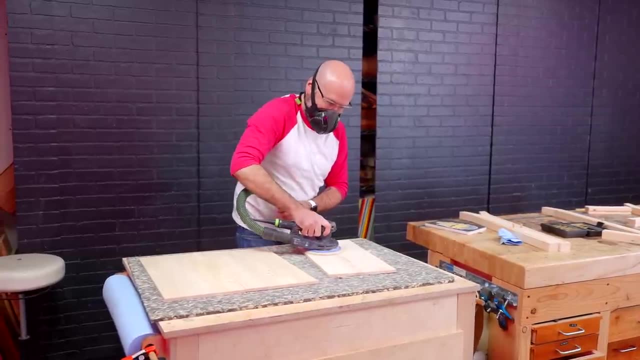 And this is probably the most important thing I'm going to do- I'm going to take the top support and the bottom support and I'm going to put them in the bottom. Then I'm going to put in the top support. The middle shelf and the bottom shelf are just going to sit on a couple of doll. 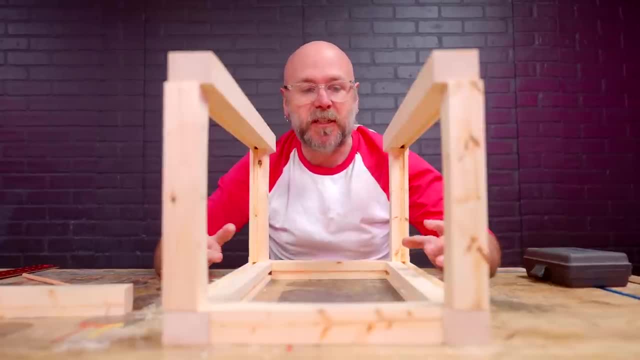 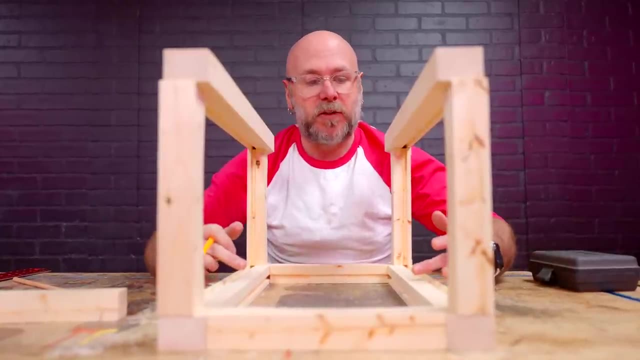 pins that we're going to cut. I don't want them permanently attached in there just because of expansion and contraction. If I was using plywood I wouldn't have to worry about that. So the middle one is going to go in optical center. 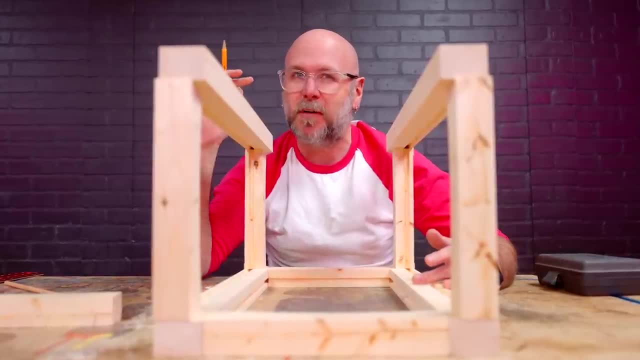 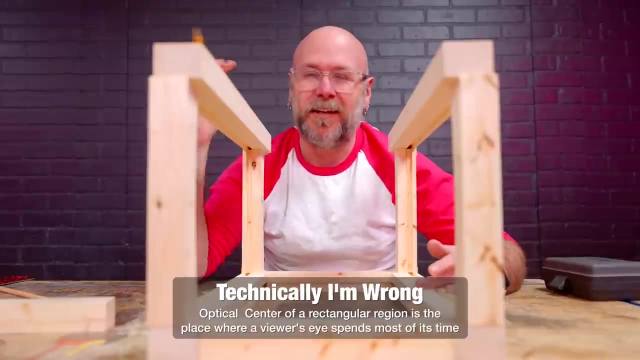 If you that's a graphic design term, meaning just above actual center, your eyes would see optical center as center. It's a. it's a whole thing. I went to school for graphic design. I ended up being a terrible graphic designer. 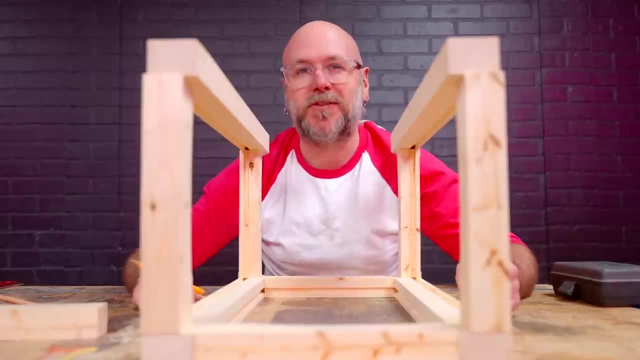 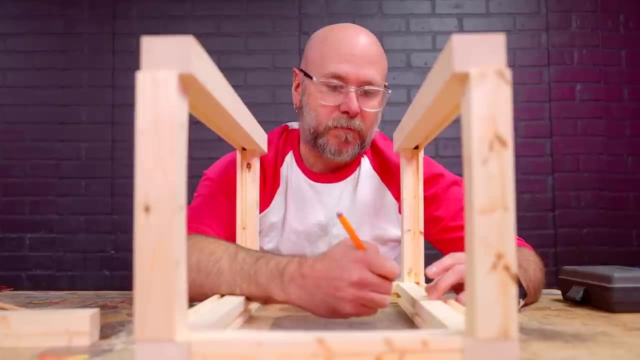 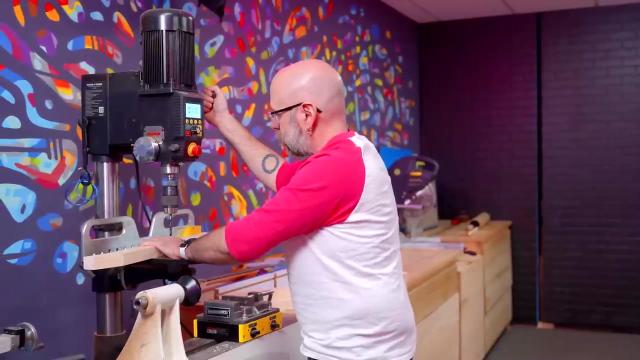 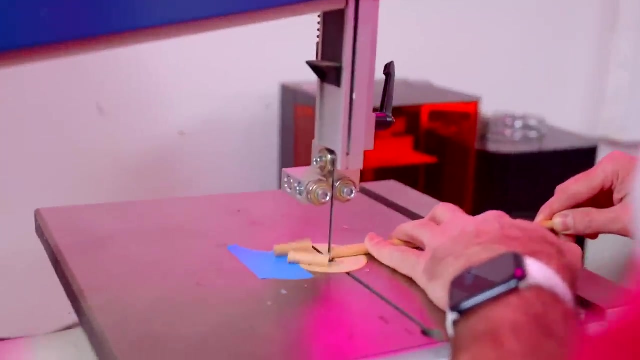 but I remember one thing from college: optical center. So, Daniel, you were a very successful graphic designer. I did Okay, I did Okay, Liar, I did Okay, Liar. All right To the drill press. So we drilled the holes. Now we found some pegs. 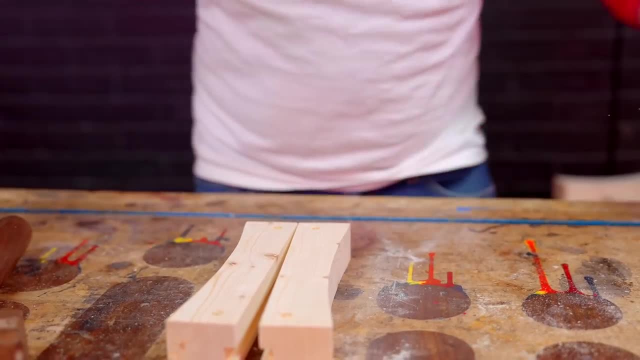 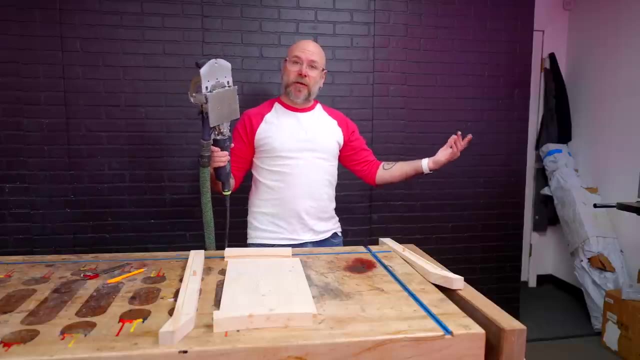 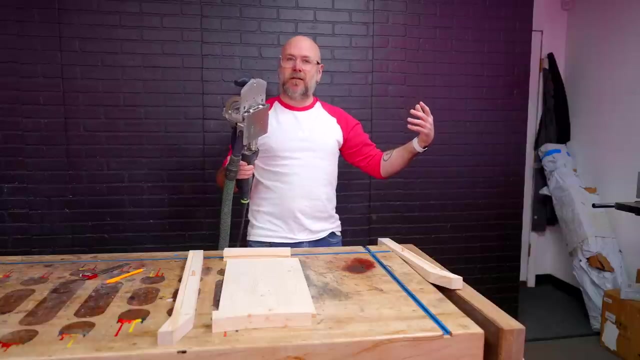 So we drilled these holes and we'll pound these pegs. Now it's time to cut the joinery so we can join things together. I guess that's why they call it joinery, Join and join. Yeah, Huh, Huh. 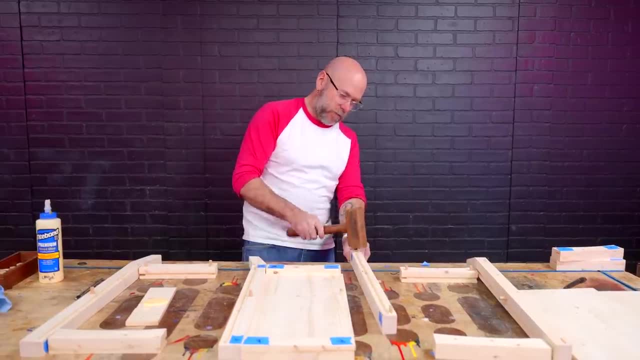 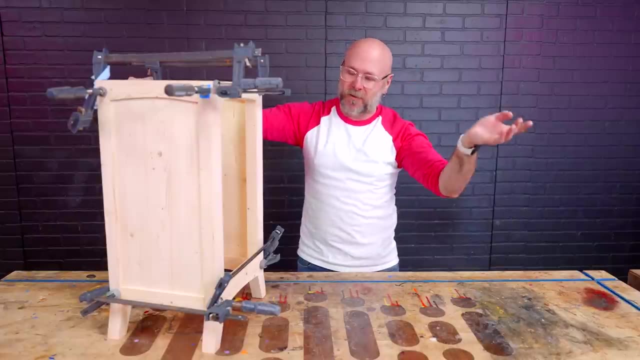 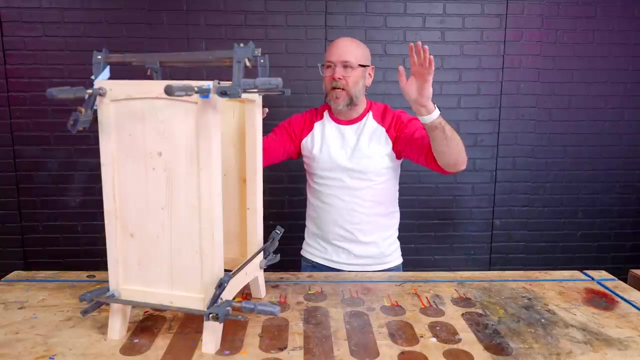 Blowing everything together and adding the Festool biscuits. I don't like sanding, I don't like finishing, I don't like using router. but I think the thing that I don't like the most, besides just woodworking in general, it's the assembly that is. it's so stressful. 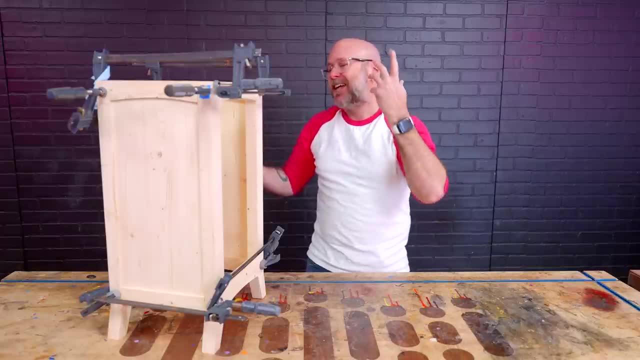 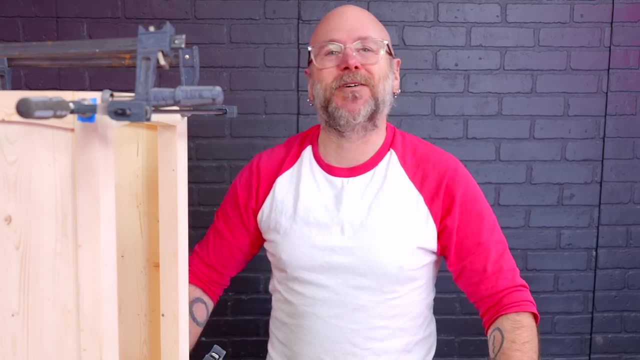 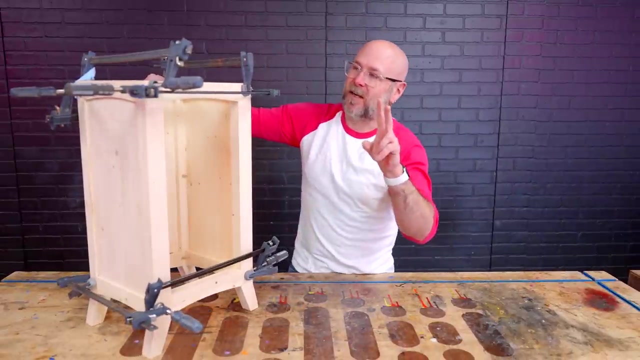 but it all goes to get like your tightening clamps and you hear things crack in and it's trying to twist and get into place And it's looking good, It's looking really good. My favorite comments- My second favorite comments- are the comments of like me using like a Festool. 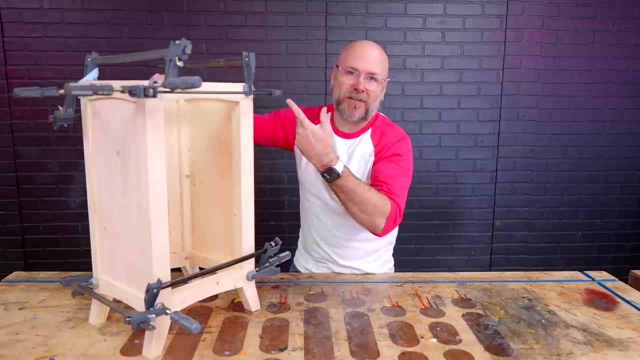 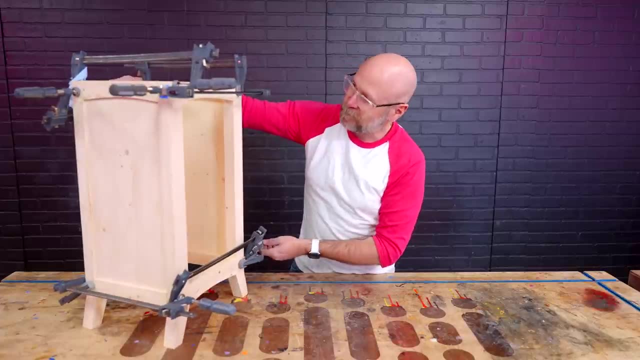 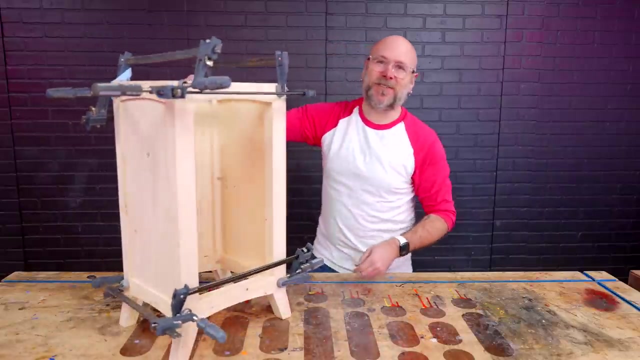 domino And then next thing, the Harbor freight clamps. People find that funny. I just, I'm just using the best tool for the job. What do you think, Dale? Yeah, Always fishing for compliments. I am very, very pleased with that. 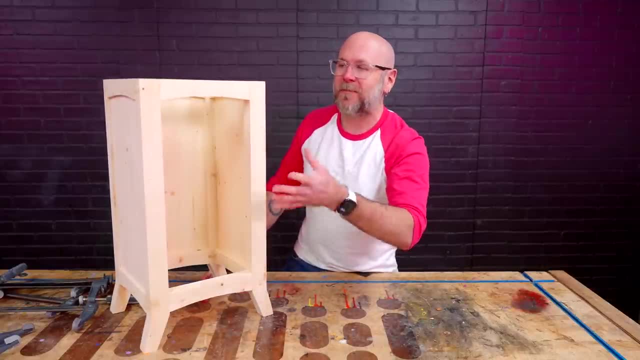 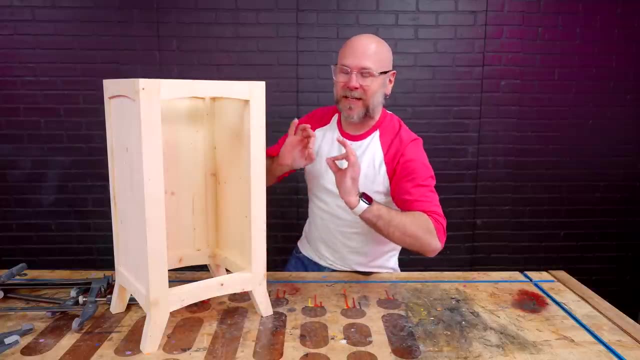 It kind of has a grandma feel. So we're going to, we're going to modernize this with some doors and the top, So let's start with the two doors. I'm going to go on here And it's going to eliminate. 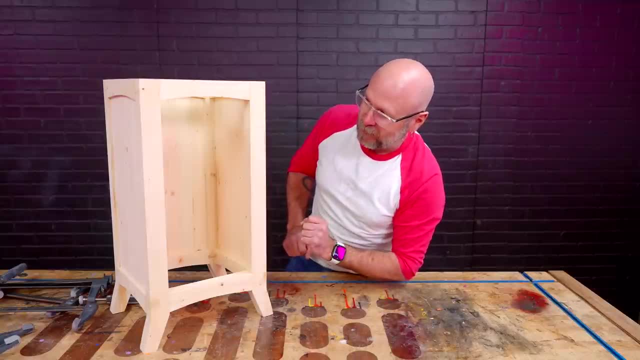 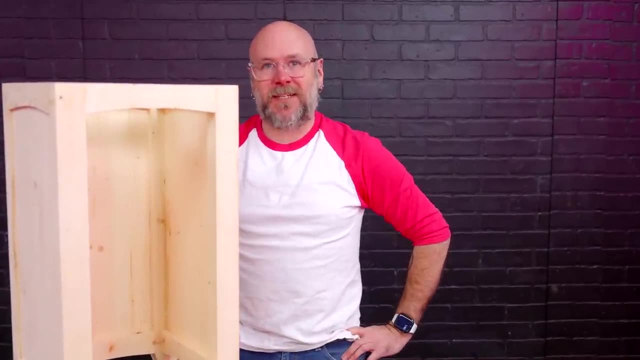 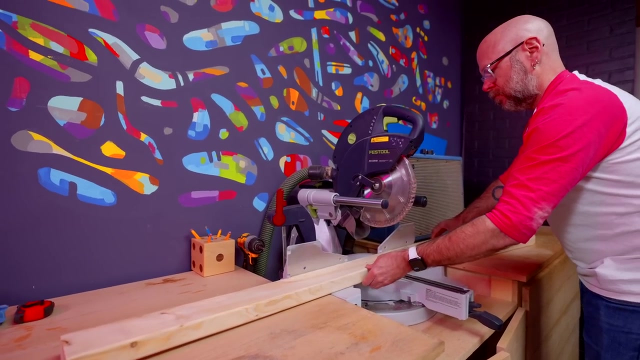 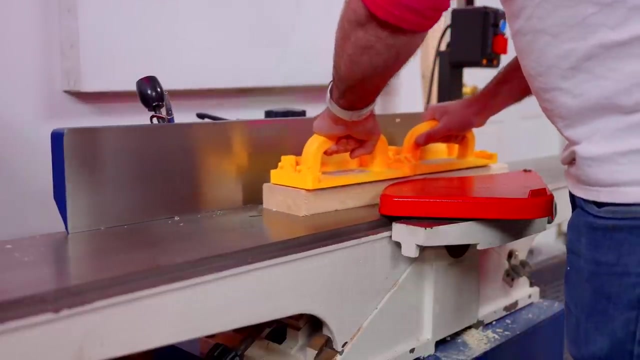 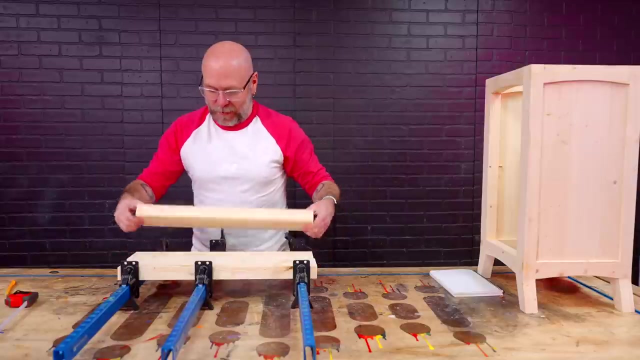 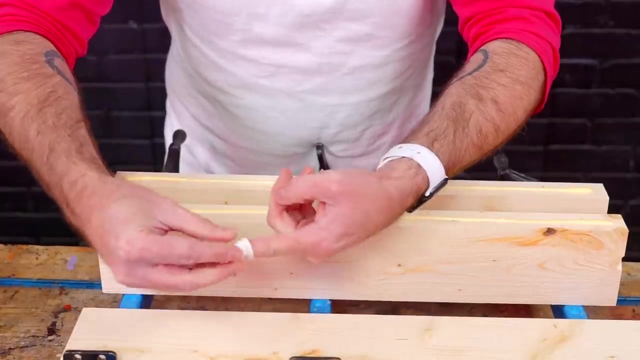 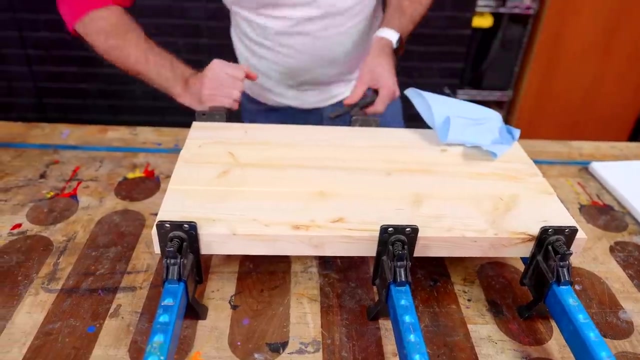 That grandma feel. no offense to grandmas out there. I love all the ladies from the eighties, the 18 eighties, All right. So got that note up. time to glue it up with some glue. Those of you who are offended by the grandma comments. I'm very sorry. 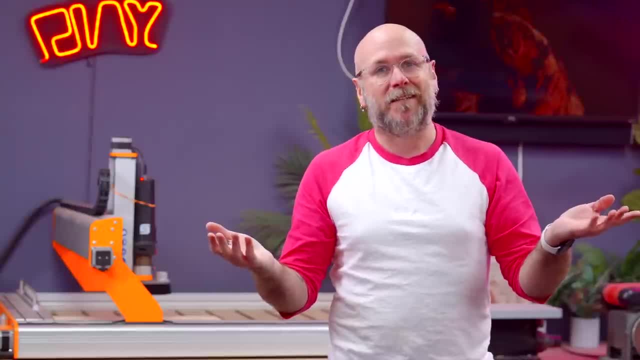 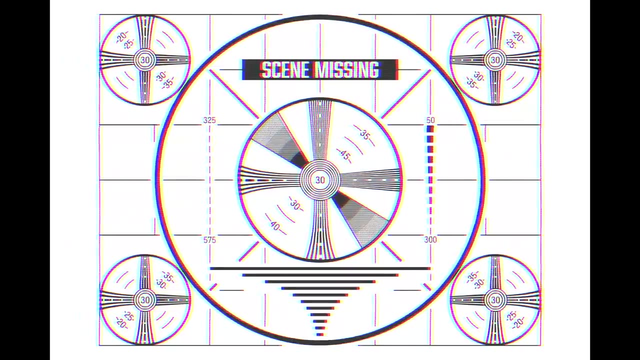 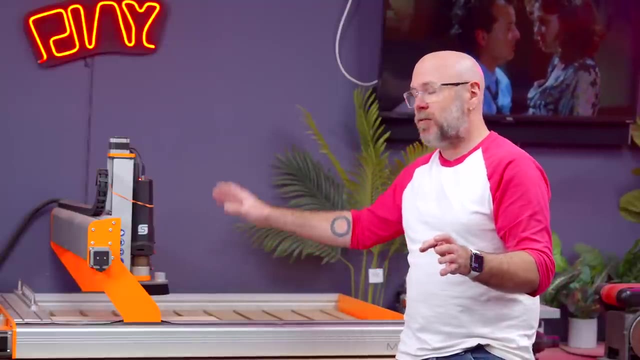 I mean no offense to your grandma, but let's be honest. If you're offended by grandma comments, maybe To get rid of the grandma ness of this cabinet I am going to carve in a design on the doors here with the step craft. 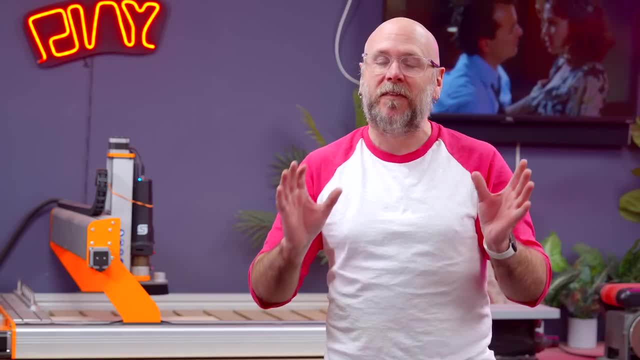 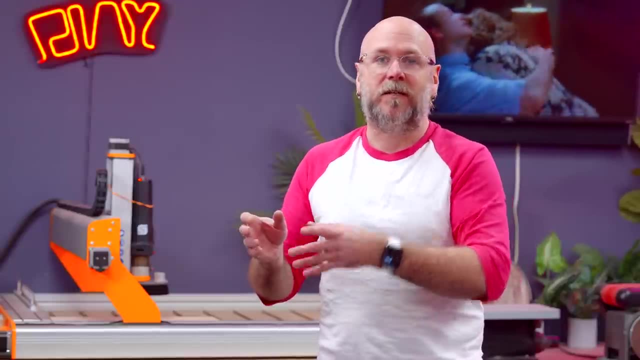 M 1000.. This is going to be a real simple pattern, but I think a lot of times simplicity is the best option. What do you think, Dale? He agrees. I'm just he he'll agree with anything that I say. 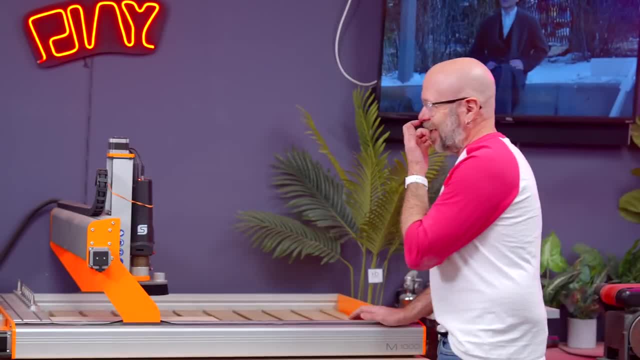 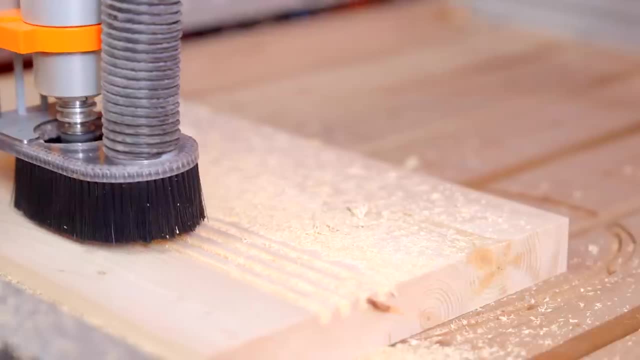 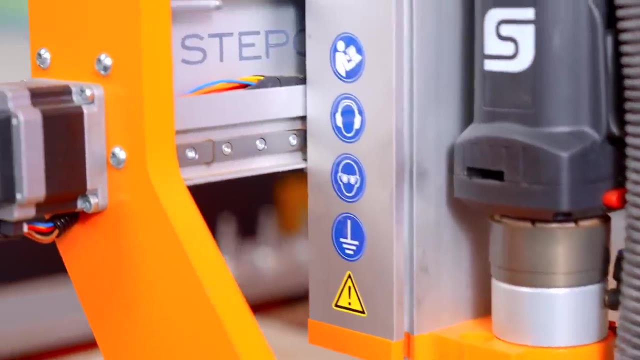 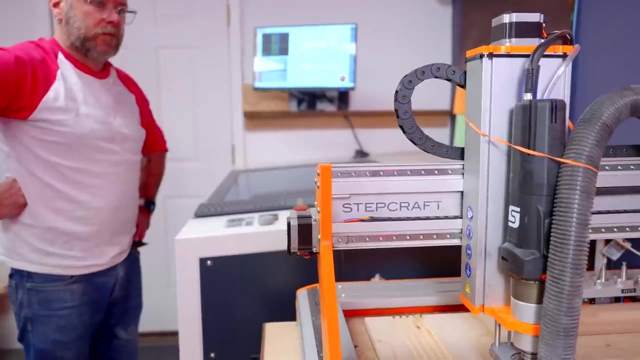 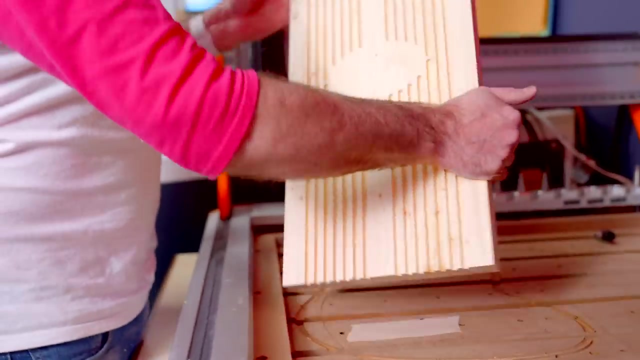 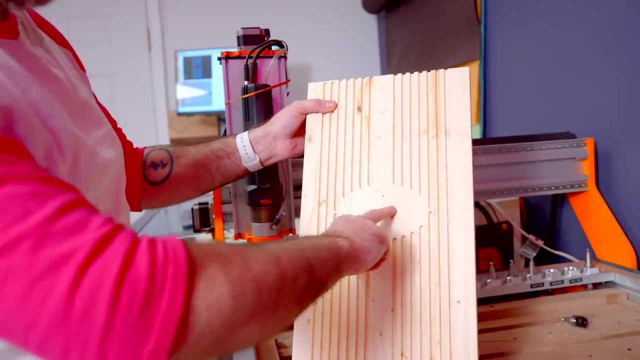 Your grandma's a whore? Were you holding that one in? All right? So now we can cut this in half. Cut that, that Ark, in there, and we'll have our two doors. We'll have a couple of nice looking knobs right there. 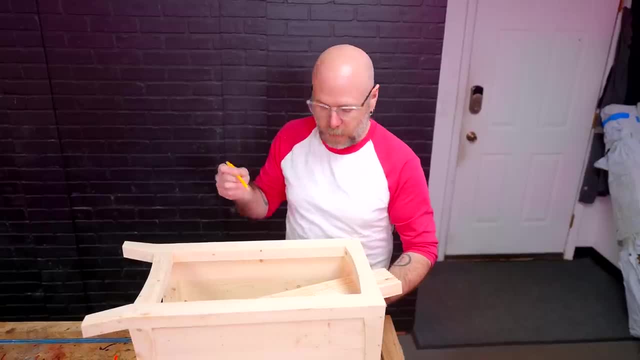 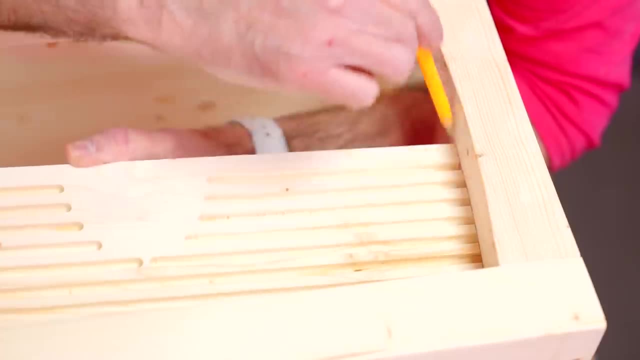 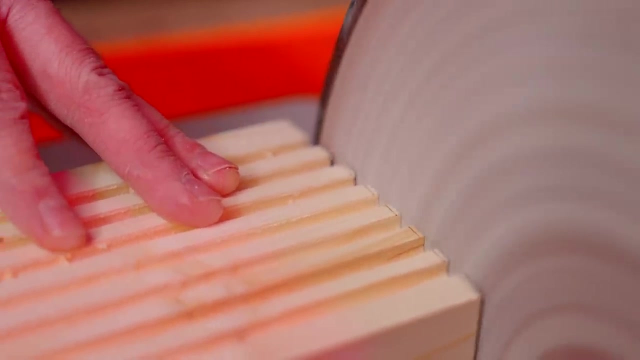 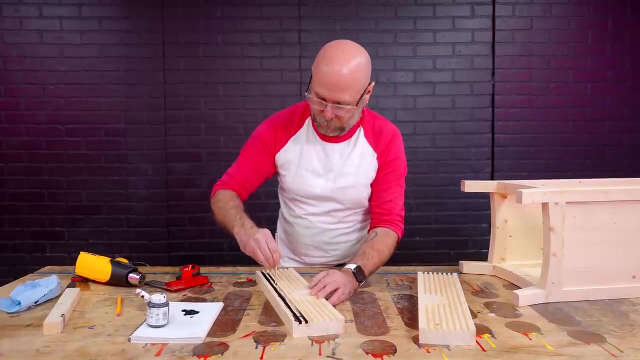 Yeah. So now I need to transfer this arc to the top of these pieces. So I'm just going to set this in here and trace that out, Paint those grooves black and then we'll sand down the top and we'll have this cool contrast. 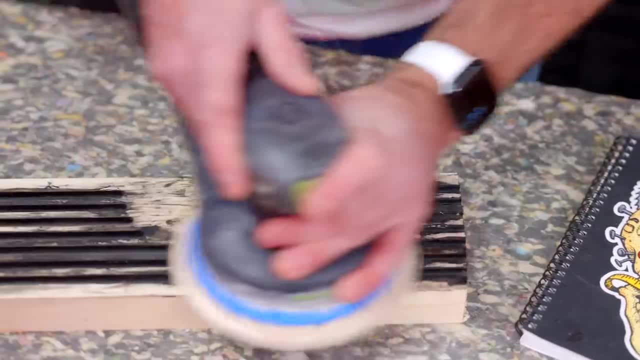 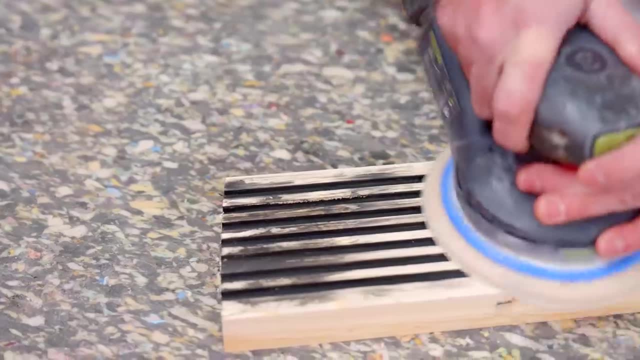 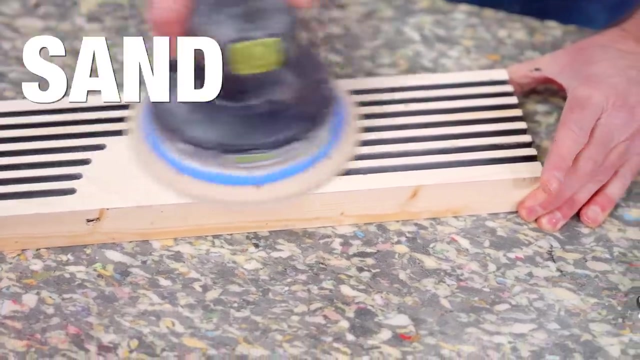 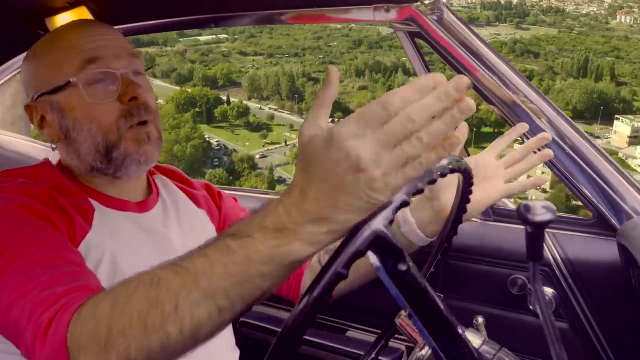 Almost done. We have to head to the store to get some dye. I want to cover up the pine and try to make it look fancy as possible, And while doing so, I'd like to tell you about today's sponsor, And that is Squarespace. I've been using Squarespace for a long time. Squarespace for like what? 10 years now, almost 10 years, way before they were a sponsor. You're probably a lot like me: You're a maker, a woodworker, an artist. 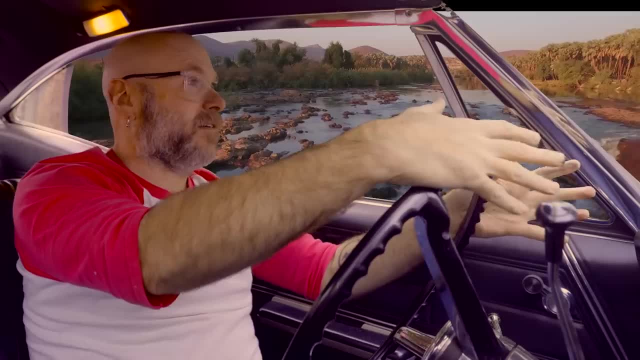 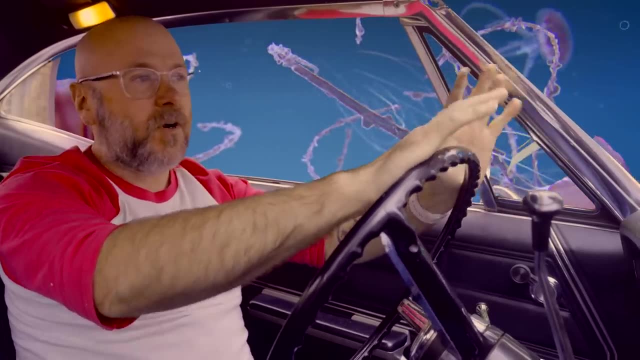 a crafter. You need a place to show up, You work, you need a place to gather clients. You need a website. Squarespace is the perfect place to do so. I've been using Squarespace so long before I was doing this full time. 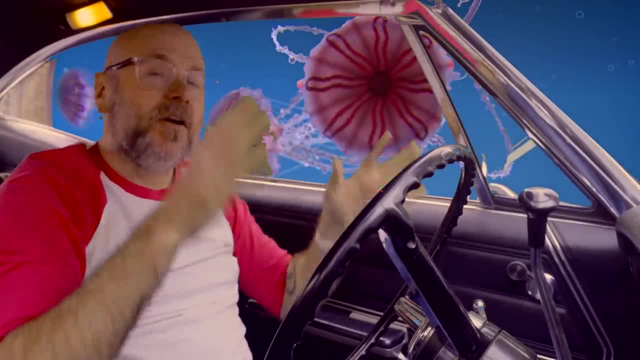 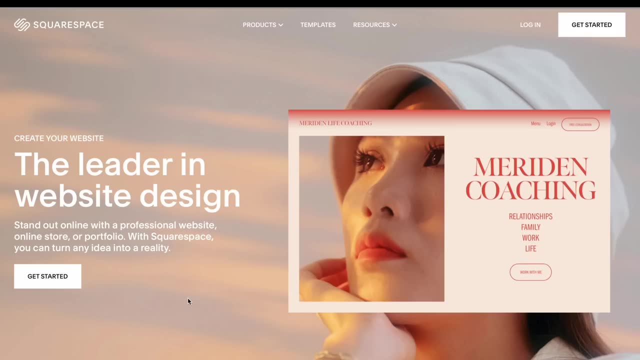 And I used to be a professional web developer. I used to sit at work all day at a computer making websites. Then I used to come home and sit at a computer all night working on freelance websites. I'm so glad I don't have to do that anymore. 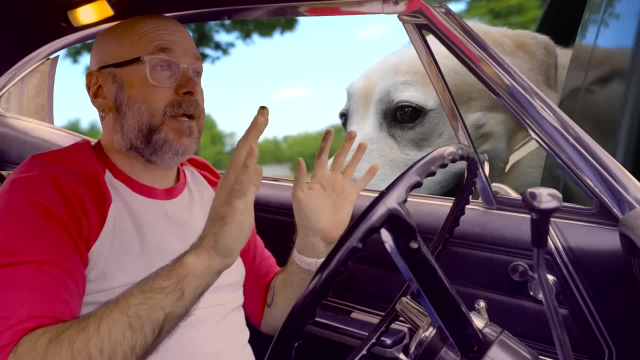 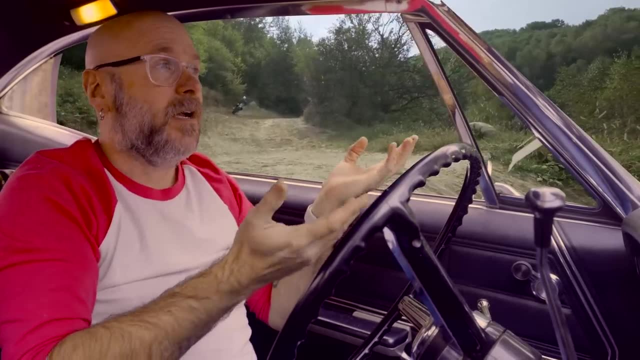 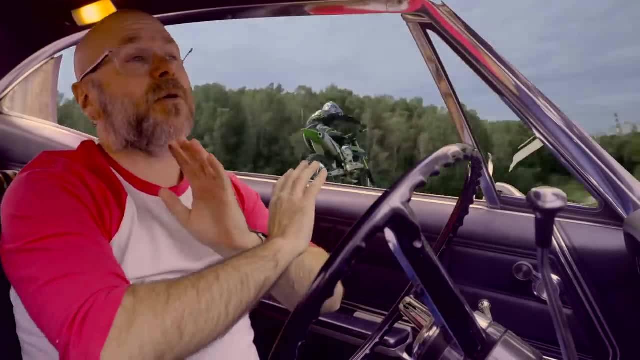 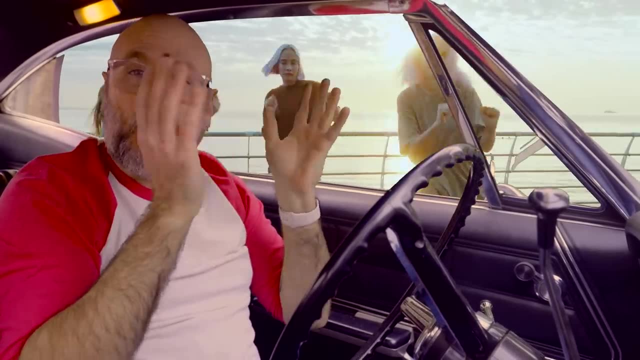 Squarespace comes in because it's super easy to set up. You don't need to know a thing about the code, cloud, backend, HTML, none of that. You can just focus on what matters to you. Galleries are easy. 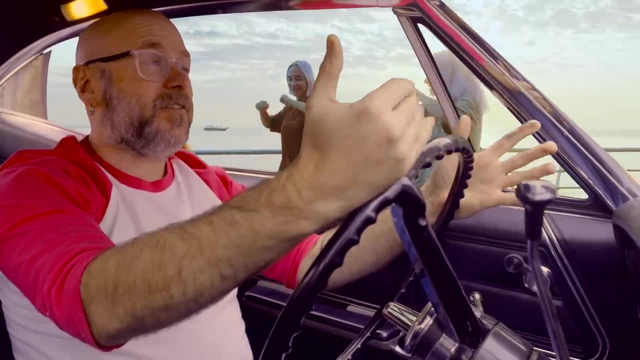 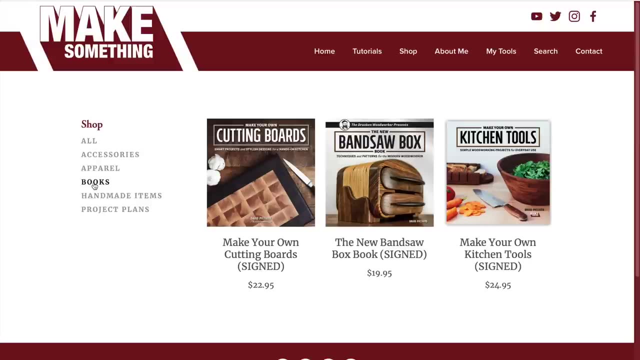 You have a number of galleries to choose from. You can sell things. You have an unlimited amount of things that you can sell on Squarespace. It just makes my life so much easier, and it can make your life so much easier as well. 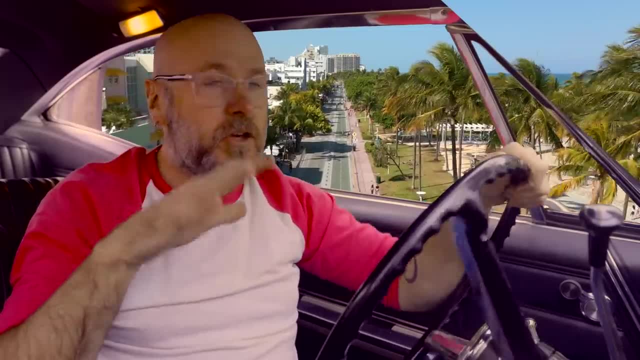 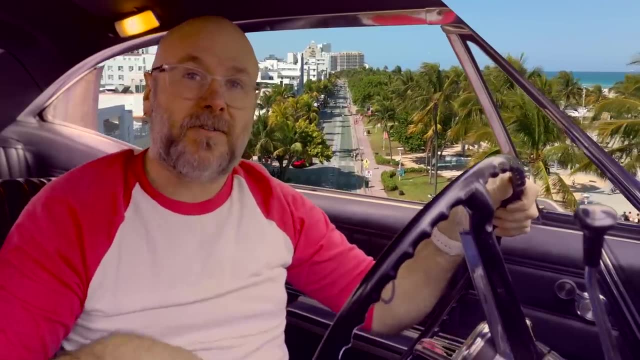 I get a lot of comments when I drive this car saying you need to wear your seat belt. You're setting a bad example. This is a 1967 Impala. It doesn't have a shoulder belt, only a lap belt. So get off my back. 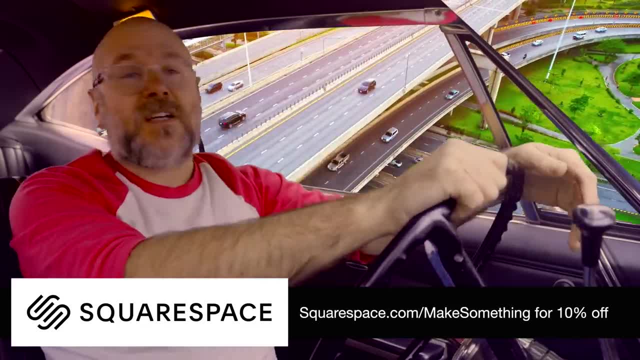 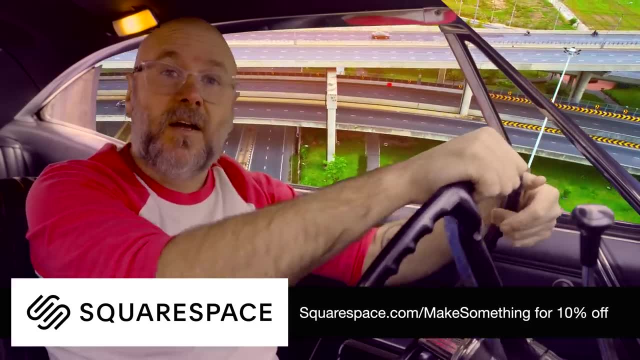 get off my back. And while you're getting off my back, visit squarespacecom. And when you're ready to launch, visit squarespacecom. slash: make something for 10% off your first purchase of a website or domain. We got our supplies. 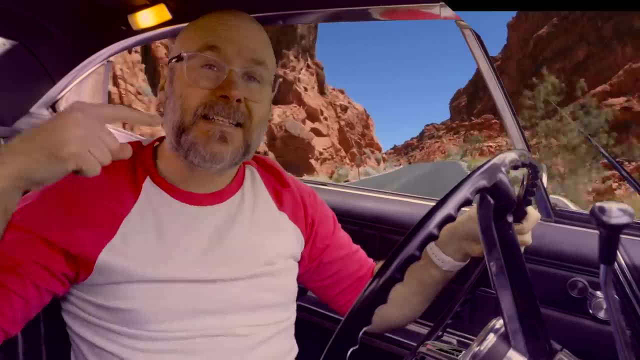 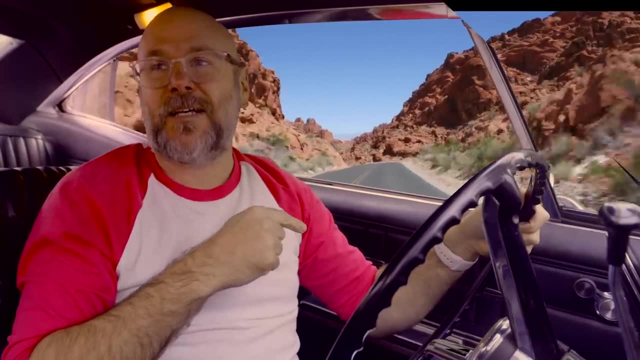 We're going to head back to the shop as fast as we can to get this finished up and just show you how freaking good this looks. It looks so good, Daniel, tell me it looks good. Are we there yet? Daniel, tell me it looks good, I will turn this car around. 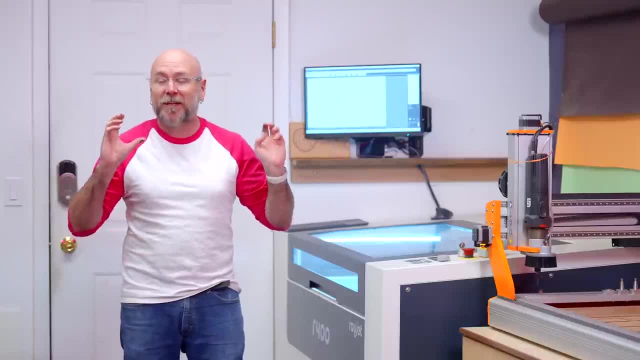 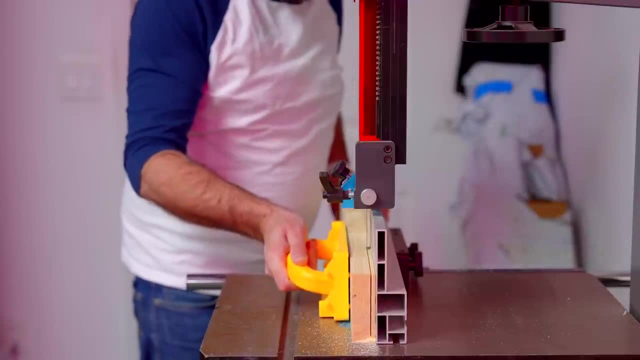 Last thing we're going to do That's really going to set This off and make it not look like two by fours, is what we're going to do for the top. I went ahead and re-sawed a whole bunch more two by fours basically into thick. 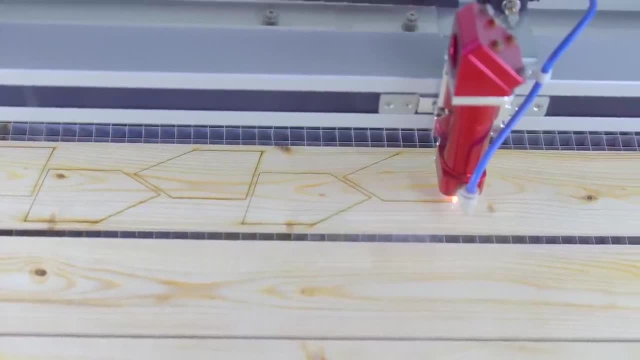 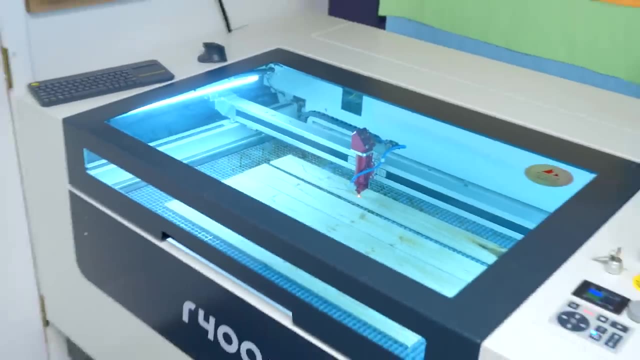 veneers And I'm going to throw them in the laser here and we're going to cut out these Pentagon. We're going to do this technique called Pentagon Pentagonal. We're going to do this technique called Pentagonal tiling And I'm going to glue all of these pieces onto a piece of plywood. 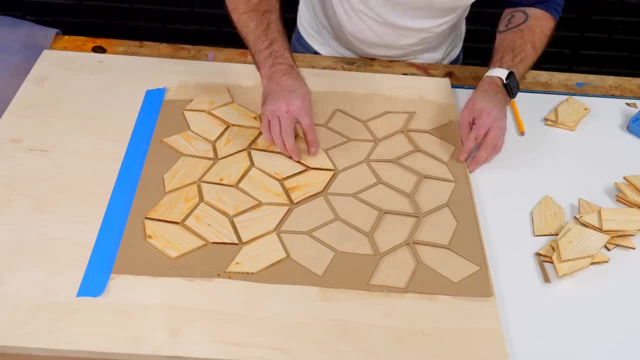 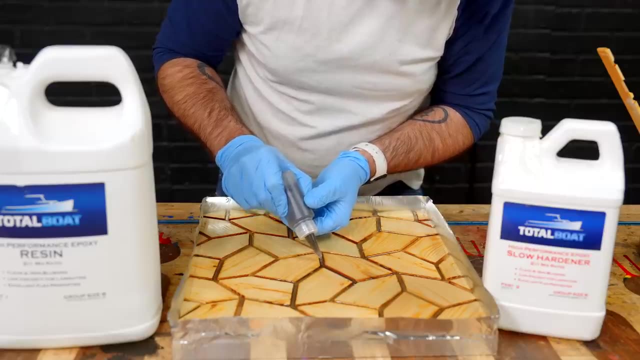 but I'm going to leave space in there and I'm going to use the vacuum bag to glue them onto the plywood And then we're going to fill that space with black epoxy which is going to match the black lines on the front doors. This is freaking cool. 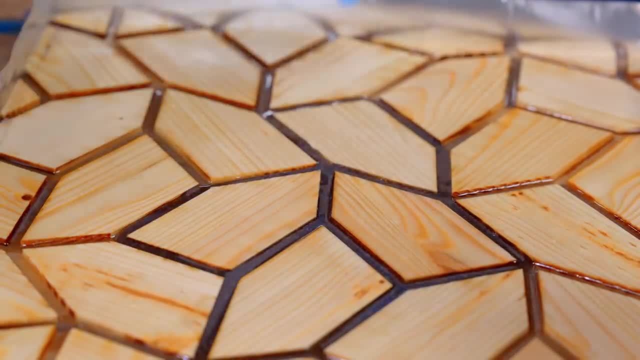 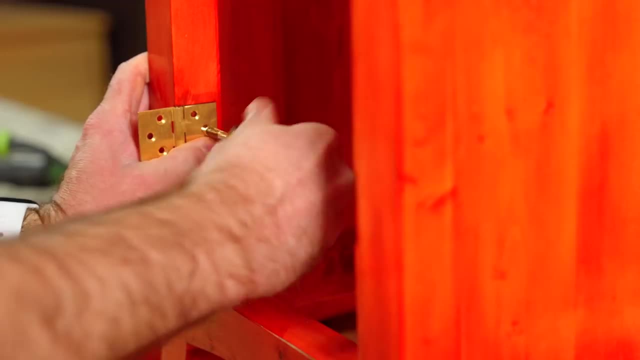 This does not look like two by fours. Holy cow, I'm blown away. I went ahead and mortised the space for some hinges, dyed everything. this cherry color added the hinges, installed the shelves, attached the top and some poles. 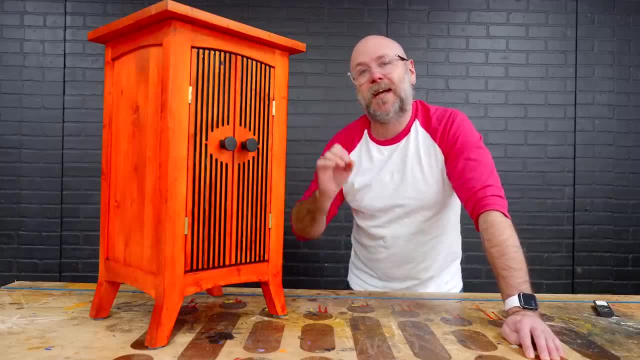 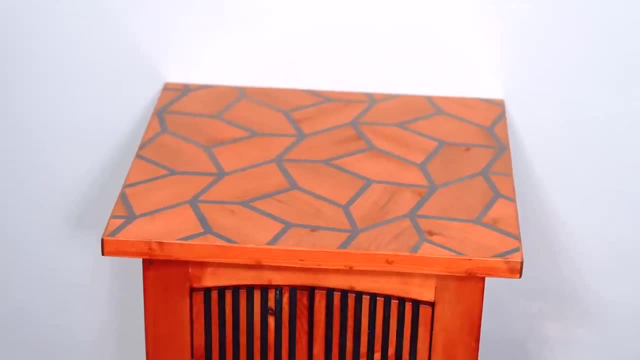 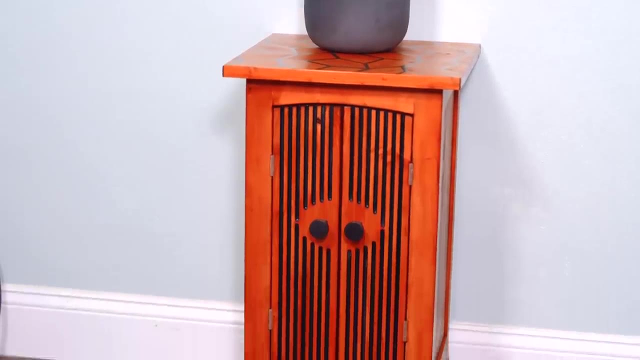 This is in direct response to all of the comments that I get saying I use Walnut way too much in my property. This is how I did this project. Anybody who enters our house and Seasons will never, in a million years, Think that this was made by two, by fours. This looks phenomenal.